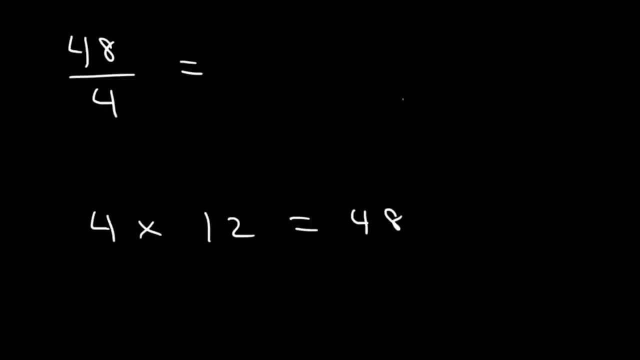 You can also use long division to get the answer as well, Whenever you need to divide fractions. 4 goes into 4 one time. Bring down the 8. 4 goes into 8 two times, and so the remainder is 0.. 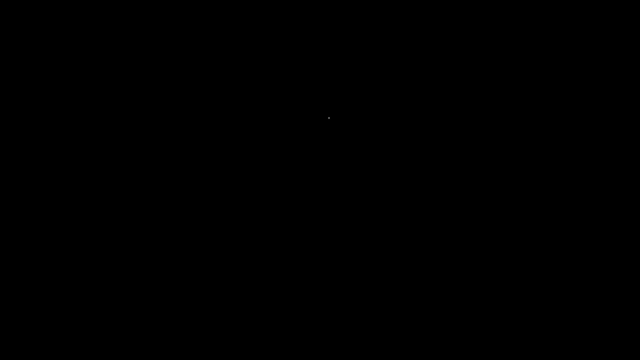 So 48 divided by 4 is 12.. Now let's review exponents. What is 4 raised to the third power? What does that mean? When you're dealing with exponents, you're dealing with repeated multiplication. 4 to the third power means that you're multiplying 3 times 4.. 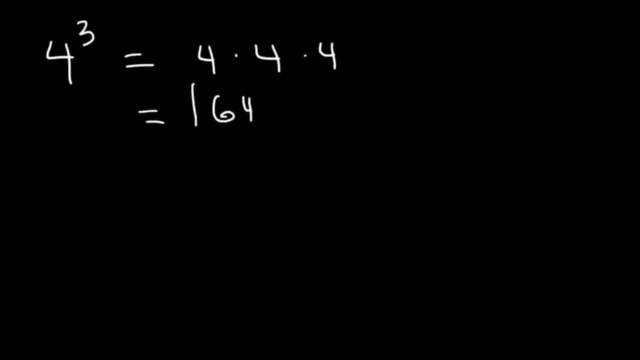 So 4 is 64.. 4 times 4 times 4 is 64.. So 5 squared means that you're multiplying 5 two times 5 times 5 is 25.. Now what is the difference between negative 3 squared and negative 3 squared? 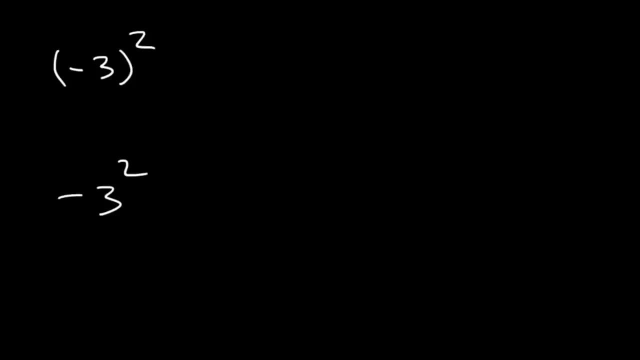 So in a typical algebra class, make sure you understand the difference between these two. Negative 3, squared in parentheses, means that you're multiplying 2 times 4.. negative 3 values A negative times. a negative is a positive number. 3 times 3 is 9.. Now negative 3. 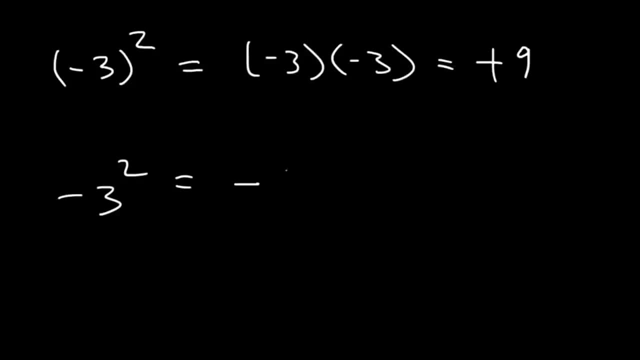 squared without the parentheses means that you have one negative sign and you're multiplying two positive 3 values. So overall, this answer is negative 9.. In addition, anything raised to 0, power is 1.. Now, when dealing with variables, when you multiply common variables, you can add: 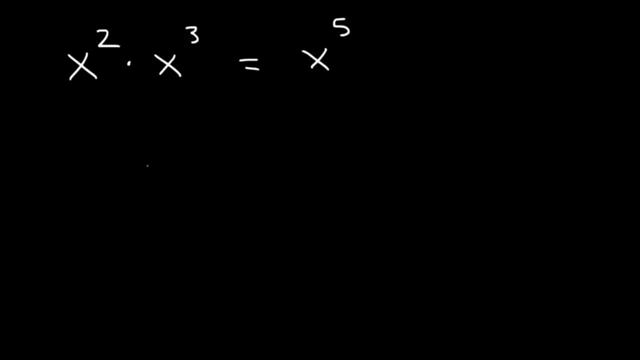 the exponents X squared times. X cubed is X to the 5th. So basically, X squared means that you're multiplying two X values, X cubed three X values, So in total you have five X variables being multiplied together. 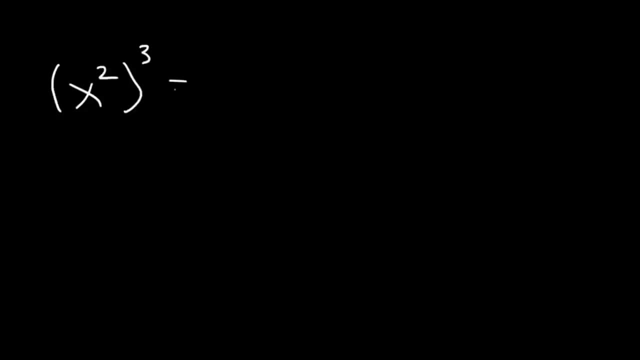 Now, what is X squared raised to the 3rd power? When you raise one exponent to another exponent, you need to multiply 2 times 3 to 6.. So this expression means that you have X squared times X squared three times, which each X squared is X times X. So in total you're multiplying six. 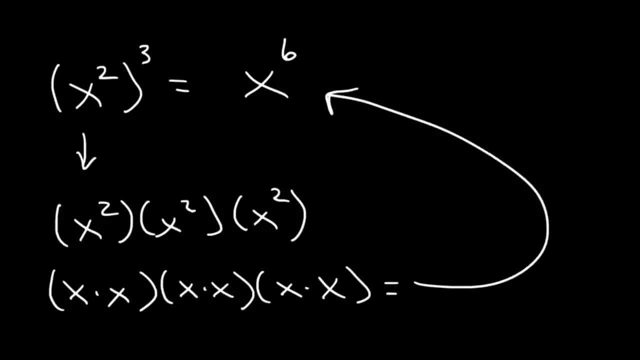 X variables, and that's why it equals X to the 6th. Now what about dividing? Let's say X to the 7th divided by X cubed, What is that equal to? So when you're dividing, what you need to do is subtract the exponents: 7 minus 3 is 4.. To 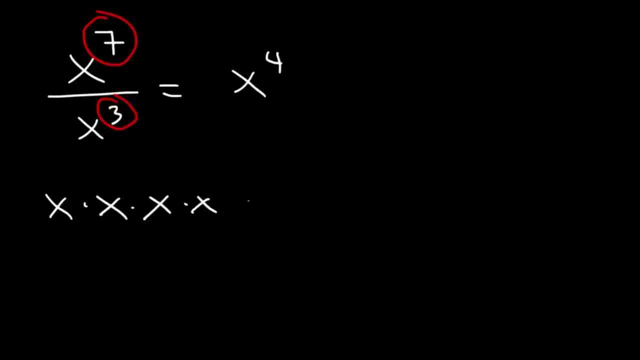 understand it, X to the 7th equates to seven X variables being multiplied together. X cubed represents three X variables. So if you cancel 3 on top and 3 on the bottom, notice that you'll have 4 left over on top. so X to 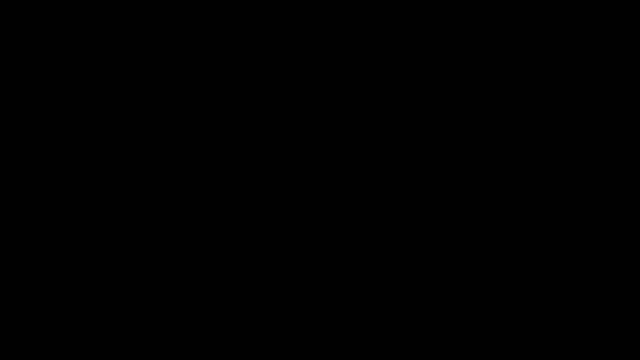 the 4th. Now you need to be familiar with negative exponents. X to the negative 3 is the same as 1 over X cubed. So if you move the X variable from the top to the bottom, the exponent changes sign. 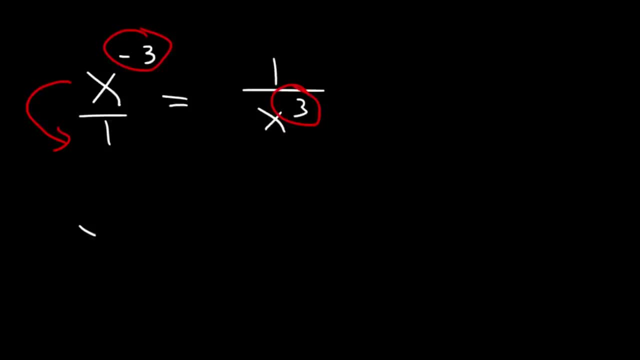 It changes from negative 3 to positive 3.. So X to the negative 4 is 1 over X to the 4th. So you can. Likewise, if you have a negative exponent on the bottom, you can move the x variable to the top and this will become positive x squared. 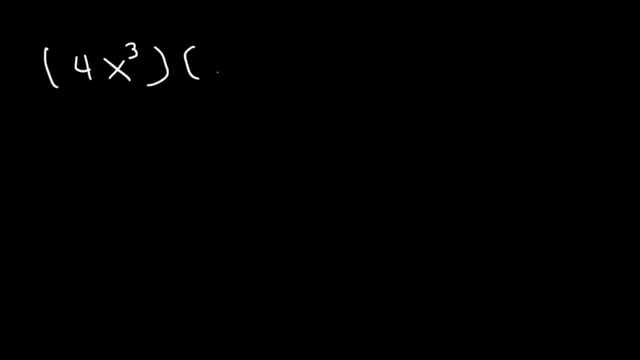 So let's say: if you want to multiply 4x cubed by 5x to the sixth, Let's multiply 4 times 5.. 4 times 5 is 20.. And then we need to multiply x cubed times x to the sixth. 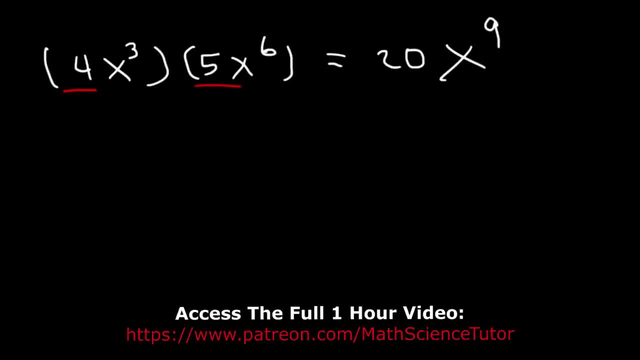 Which we need to add 3 and 6, that's 9.. So it's 20x to the ninth. So go ahead and work on these examples: 5x to the fourth times, 3x to the seventh And 24x to the eighth, divided by 6x to the fifth. 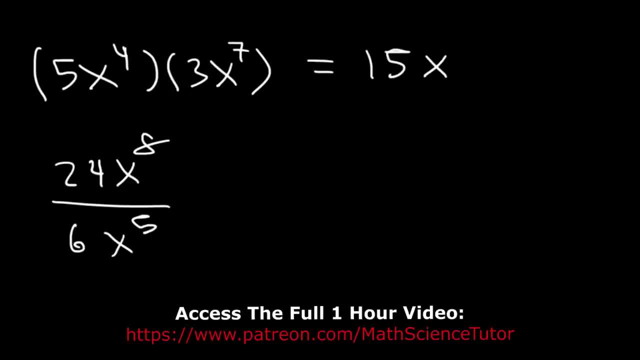 So 5 times 3 is 15.. And x to the fourth times 3x to the seventh. We need to add 4 plus 7.. So that's 11.. Here we need to divide 24. divided by 6 is 4.. 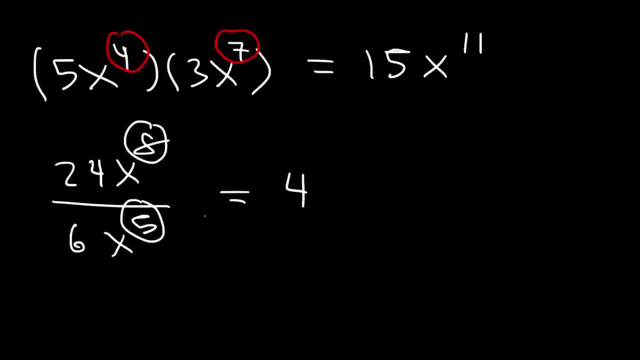 And x to the eighth divided by x to the fifth, We got to subtract 8 minus 5.. So it's 3.. So you get 4x cubed. Here's another example. Simplify this expression: 28x to the fourth divided by 4x to the sixth. 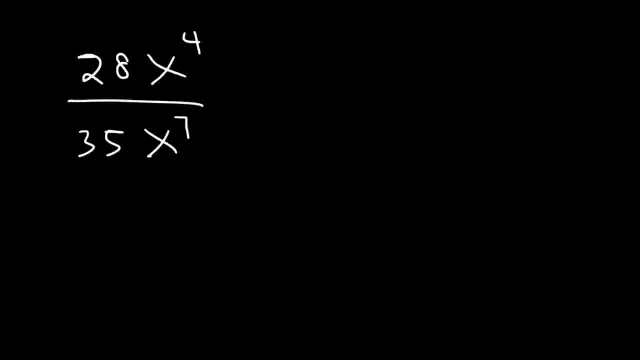 And now we'll multiply it by 35x to the seventh. Feel free to pause the video Now. in this example, I'm going to break down 28, into 7 and 4.. 35,: I'm going to break it down into 7 and 5.. 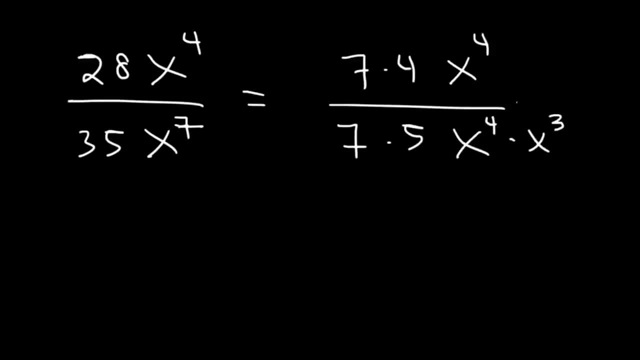 x to the seventh. I want to write it as x to the fourth times x to the third, Because 4 plus 3 adds up to 7.. So I'm going to multiply that 7.. Notice that I can cancel a 7, and I can cancel x to the fourth. So the final answer is 4 divided. 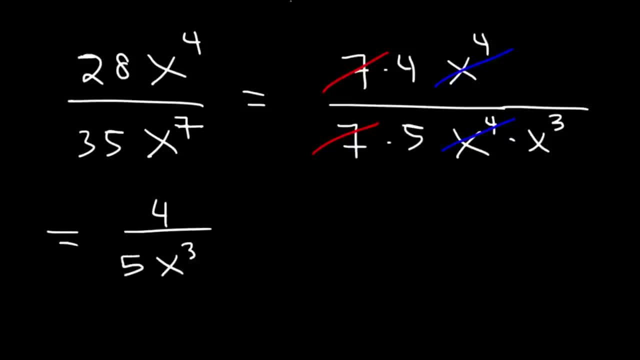 by 5x cubed. Now, granted, you could have subtract 4 and 7. 4 minus 7 is negative 3. Now it's x to the negative 3 on top, but if you move it to the bottom it becomes 1 over x cubed. So in the end, 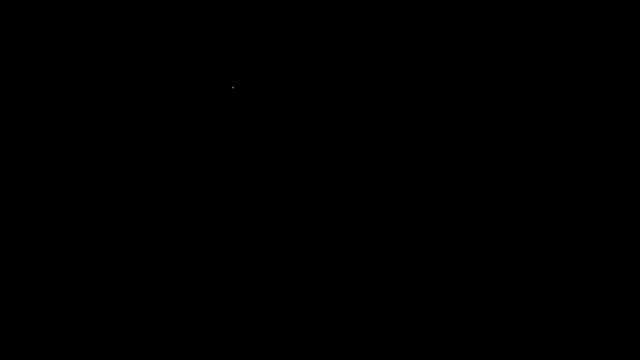 you should have x to the third on the bottom. Here's another example that's similar. Let's say we have 63x to the fourth, y to the third, over 56x to the eighth, y to the fifth. 63 is 9 times 7, and 56 is 8 times 7.. x to the eighth is x to the fourth times x to the fourth. 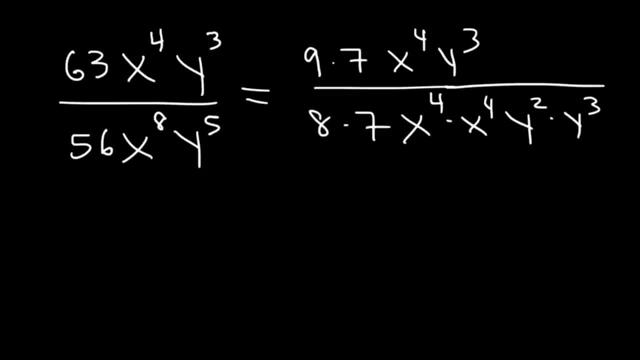 y to the fifth is y squared times y cubed: 2 plus 3 is 5,, 4 plus 4 is 8.. And then I'm going to cancel the 7, I'm going to cancel x to the fourth and I'm also going to cancel y cubed. So my final 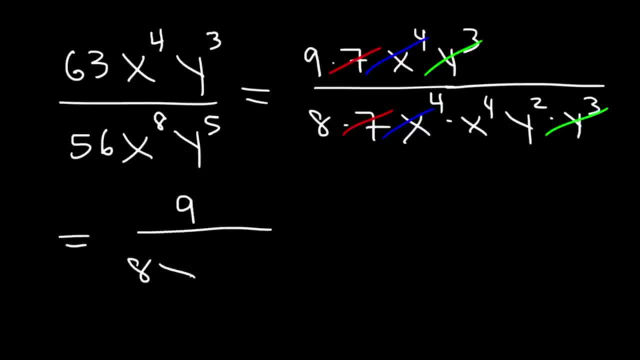 answer is 9. divided by 8x to the 4th y squared. So that's the nicest simple way to simplify expressions that look like that. Now, sometimes you may have to deal with exponents. Let's say we have 2x cubed. 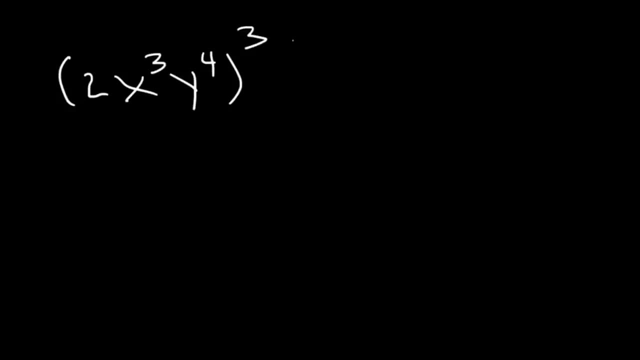 y to the 4th, raised to the 3rd power. How can we simplify this expression? So when you raise one exponent to another, you need to multiply. So first we're going to multiply 3 by 1.. 3 times 1 is 3.. And then 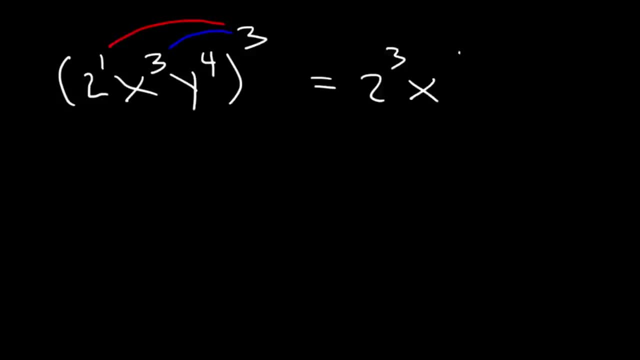 3 times 3,, which is 9.. And 4 times 3,, which is 12.. 2 to the 3rd power means that we're multiplying 3- 2's together. 2 times 2 times 2 is 8.. 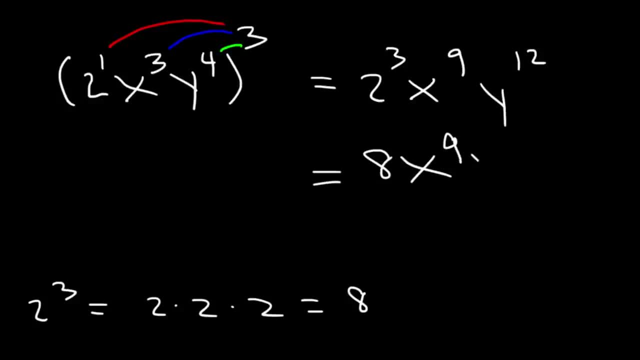 So the final answer is 8x to the 9th y to the 12th. Try this one: 3x squared y to the 3rd raised to the 2nd power times. 4x cubed y to the 4th raised to the 3rd power. 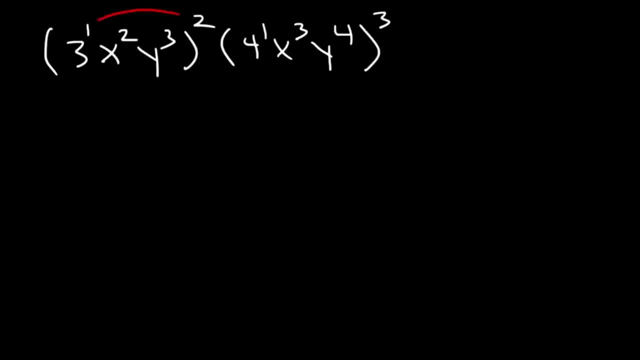 So let's distribute 2.. 2 times 1 is 2.. So we're just going to have 3 squared, y to the 3rd power, 3 squared, And then 2 times 2 is 4.. So that's going to be x to the 4th. 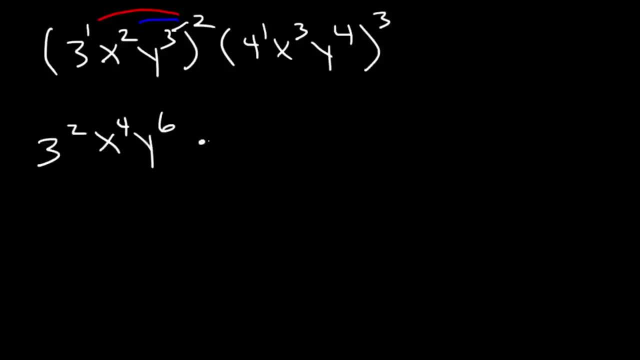 And 3 times 2 is 6.. And then we have 3 times 1,, which is 3.. And then 3 times 3,, that's 9.. And finally, 3 times 4 is 12.. 3 squared is 3 times 3.. 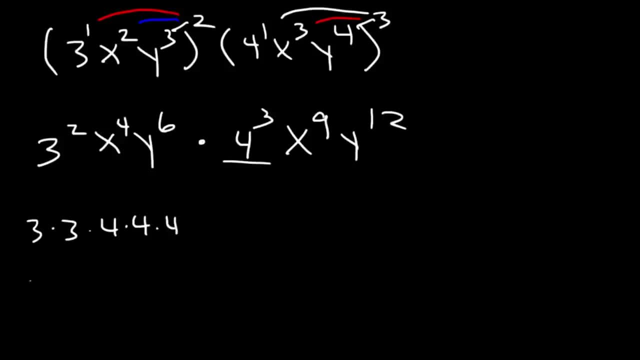 4 cubed is 4 times 4 times 4.. x to the 4th times 3 is 4.. x to the 9th, we need to add 4 plus 9.. So that's 13.. And y to the 6th times y to the 12th. 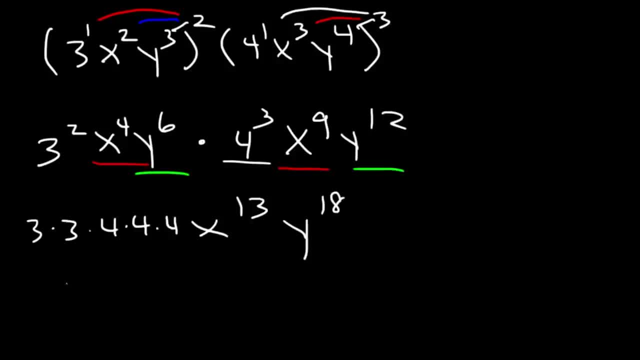 we have to add 6 and 12,, which is 18.. Now, 3 times 3 is 9.. 4 times 4 times 4 is 64. So what is 9 times 64?? If you don't want to use a calculator,